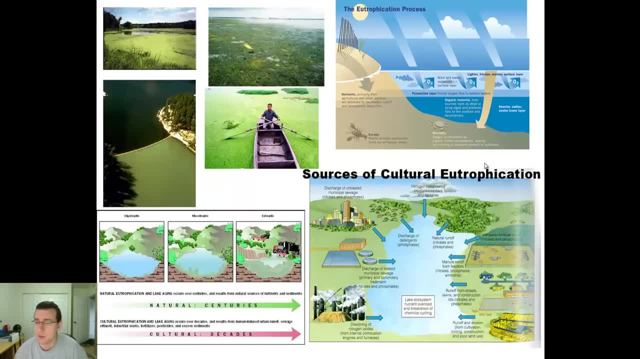 The other interesting pattern of growth that's actually important for population ecology is the idea of nutrient limitation versus nutrient excess. Remember that how much carrying capacity you're going to have depends on the availability of nutrients that exist in the ecosystem. So if the nutrients are very limited for the producers, the productivity is going to be low and the carrying capacity is going to be very, very low because there's not a lot of producers doing their jobs. So that can't maintain a very large pyramid of energy. Remember we talked about that on the very first topic. 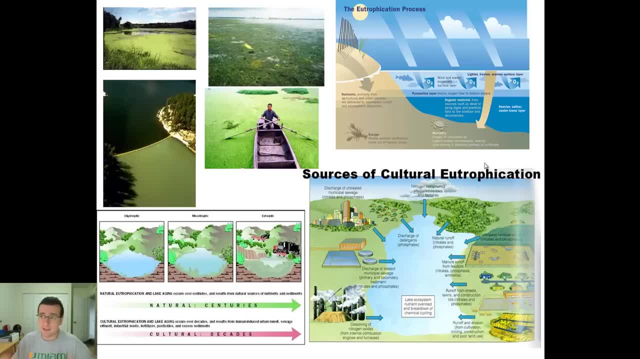 But if the opposite happens and all of a sudden you have an excess of nutrients, that means that the producers can explode and produce as much as they possibly can. Now that seems like a good thing for the ecosystem, because now you have a lot of producers and all of a sudden you can have awesome, awesome amounts of life. But that actually can have detrimental effects to the food web. For starters, if you have an excess of productivity, everybody's going to want to eat all those producers. It's going to send cascade effects of bottom-up control. 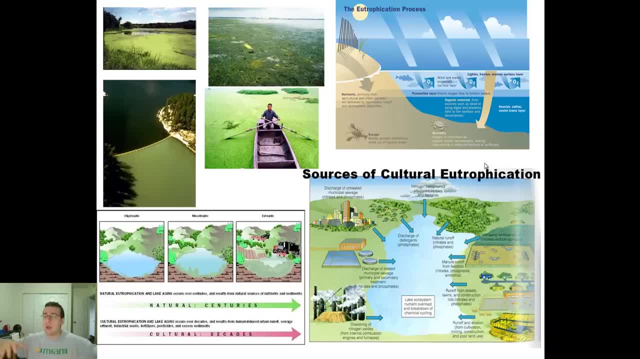 There's going to be so much food at the bottom that the whole food web now can grow. Everybody can grow at once, pretty much, But in those kinds of circumstances- the animals which are better adapted for the environment, the more competitive animals, the ones which are more dominant- they will tend to overcompete everybody else for those new resources and it will actually decrease the biodiversity of the food web because of that. So too much productivity can actually hurt the food web sometimes. 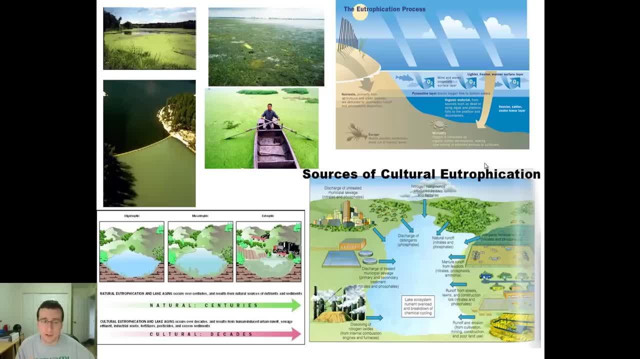 All right. The best example of that actually is the process of eutrophication. That's what you see in the screen over here Now. eutrophication happens in natural lakes and we already talked about it when we did ecosystem ecology. But here I'm showing you again the kind of idea of what's going on Now. basically, the lake, it's the very beginning of its life. It's called an oligotrophic lake. It's a clean lake. It barely has life living in it. It doesn't have too many nutrients gathered on the side of the lake. But throughout the lifetime of the lake, animals living in the lake, organisms living in the lake- they're all living in the lake. 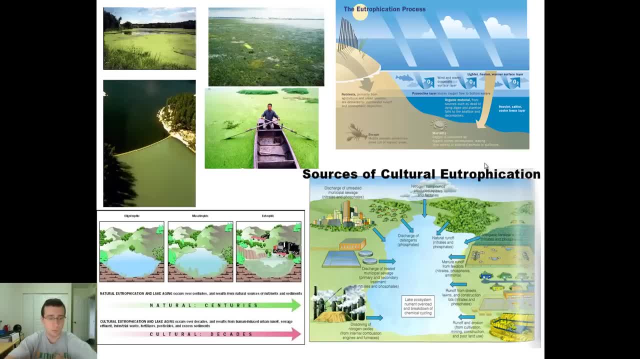 The lake will die off and they will settle to the bottom or it will be decomposed by decomposers. Meanwhile, rain and runoff from areas around the lake are carrying even more nutrients inside the lake. So throughout the life of the lake, both because the lake itself, the life of the lake itself, is dying and because runoff from the outside is actually adding more, the lake will actually increase its level of nutrients inside the lake. Now remember, the more of these nutrient levels increases, the more productivity it will have. 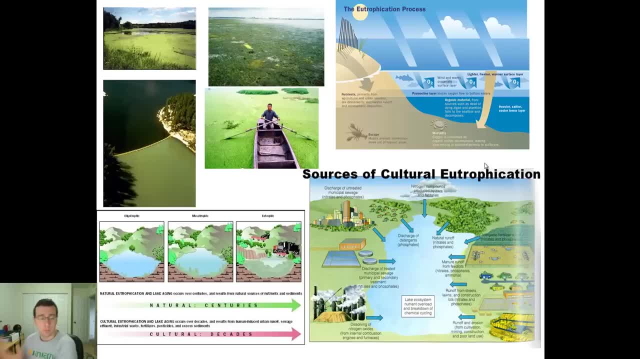 It can actually occur, The more decomposition will occur and then the more productivity will follow And the lake, throughout time, will become more and more nutrient rich And the bottom of the lake will become more and more filled with that detritus- that's what we call the dead stuff that lives in the bottom. So you'll go from oligotrophic to mesotrophic and finally to eutrophic, which is the final stage of the life of the lake. Now, on this final stage, what happens is what you see in the pictures on the top left, which is roughly a representation of the life of the lake. 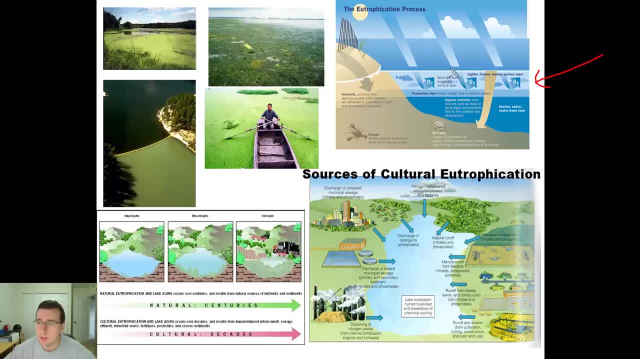 This diagram on the top right. Light from the sun will continue to hit the surface of the lake where the warm layer, where all the producers will try to live, And that layer will be very, very oxygenated because the producers are living there constantly doing photosynthesis and adding oxygen to the layer. But then this excess of producers- there's so many of them that everything that lives dies. So eventually those producers will die off and sink to the bottom of the lake where they will gather as even more nutrients. 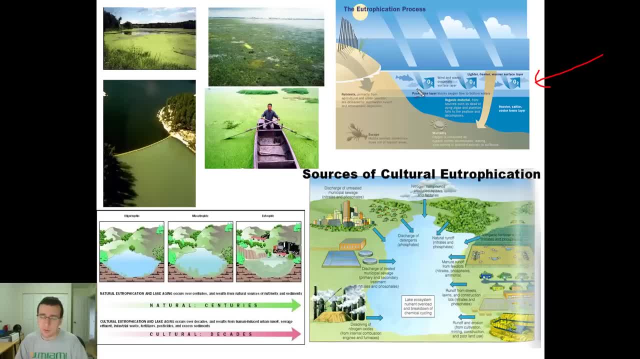 So with time it gets so saturated with nutrients in the bottom, the decomposition will increase more and more because more and more dead stuff is gathering. The decomposers that's living in the bottom will go crazy. It's like a feast of decomposition. But decomposition produces carbon dioxide and other toxic gases And actually the nutrients will actually gather to toxic levels in the bottom of the lake And it's going to get saltier down there. It's going to be cooler because the sunlight starts to be blocked by all those producers. 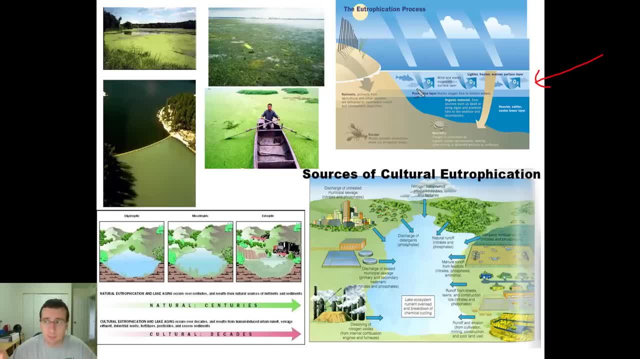 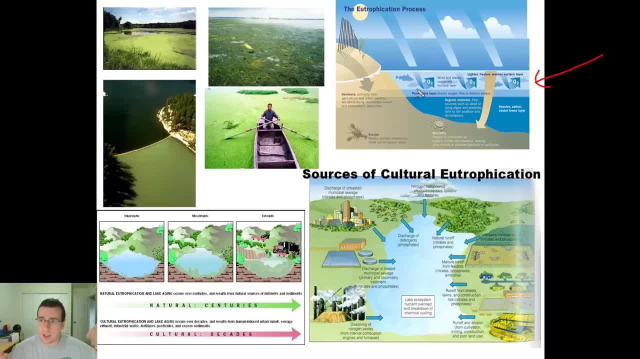 the photic layer is actually going to block the flow of oxygen into the lower water, and when you get to that point, life in the bottom of the lake becomes impossible because it becomes air deprived. so even everything that lives down there will die off because they are going to be unable to breathe. 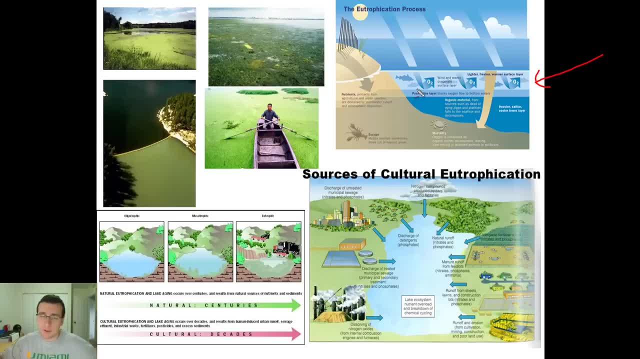 down there. so all you have left is a layer of productivity on the top in a dead lake on the bottom. now, this will continue for a long time until, finally, even the producers themselves will start to start from oxygen and become toxified by the water, and then the lake will actually finish. 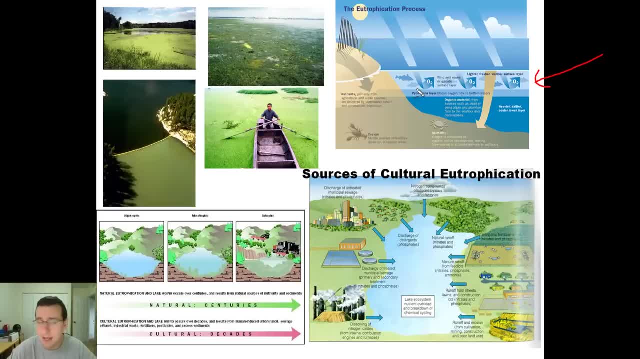 with a thin layer of produces on the top in a dead, dead detritus lake in the bottom. that is a gentrification process and it does happen naturally. over centuries, the lake actually becomes more and more neutral nutrients. however, unfortunately, cultural gentrification is increasing. 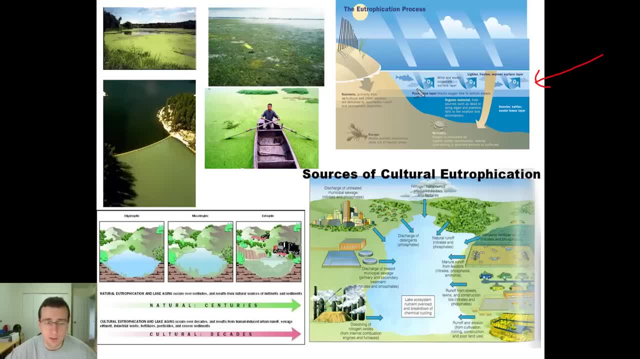 lately. it starts from sewage discharged from untreated sewage from the cities or treated sewage, nitrogen coming from from acid rain and other things like that. discharge of phosphates for plantations and nitrates and phosphates from natural sources. manure runoff from all the things that, all the animals that. 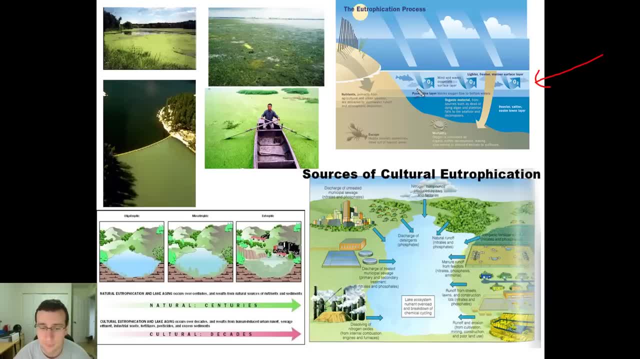 we grew the growing inorganic fertilizer like nitrates and phosphates, which are being added to the lawns of people, erosion and runoff from cultivation, from areas of construction and all other kinds of stuff that we do are constantly going to be adding more and more. 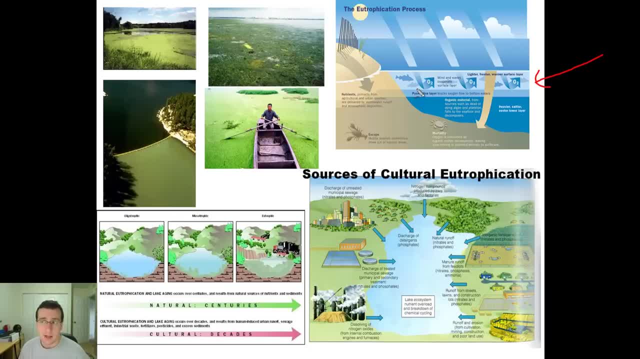 nitrates and phosphates to the water of these lakes, and then that makes the eutrophication process speed so much that, instead of taking centuries, it will happen in just a few decades. and then the lake will go from oligotrophic to eutrophic or the dead lake in a matter of years.